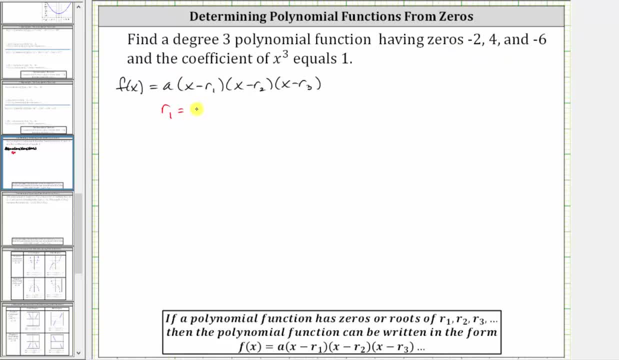 So let's let r sub one equal negative two, r sub two equal four and r sub three equal negative six. And because the coefficient of x cubed is equal to zero, we are asked to find the root, or roots, of a polynomial function. 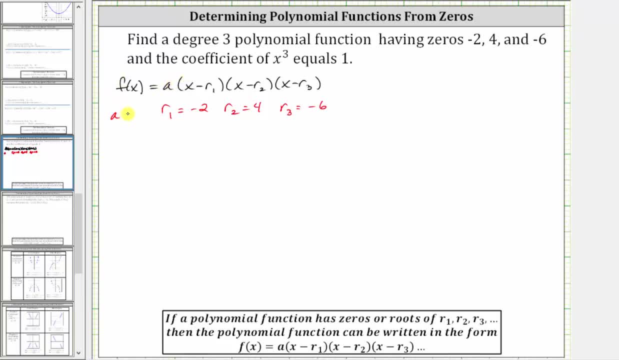 And because the coefficient of x cubed is equal to one, we also know a is equal to one, which means a polynomial function that satisfies the given conditions will be: f of x equals one times the quantity x minus negative, two times the quantity x minus four times the quantity x minus negative, six. 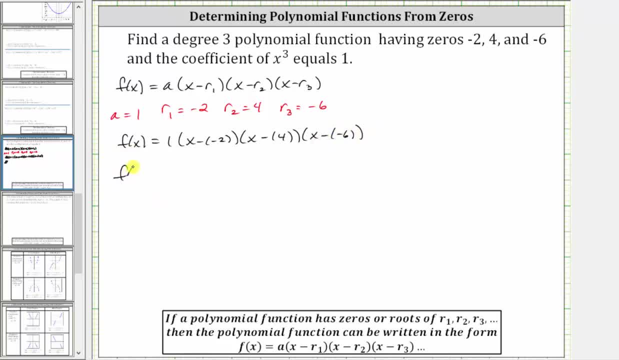 And now let's simplify the right side. We have f of x equals. multiplying by one doesn't change anything. x minus negative two simplifies to x plus two. then we have x minus four and x minus negative six simplifies to x plus six. 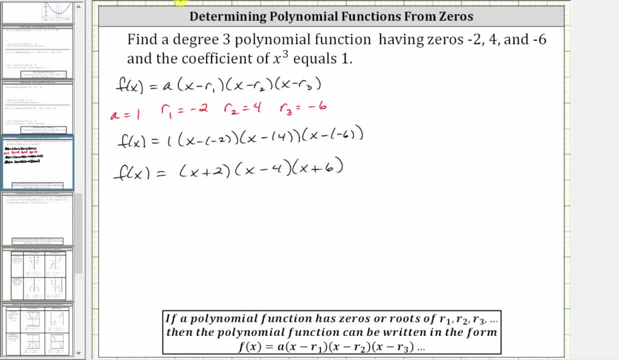 So this is the factored form of a polynomial function that satisfies the given conditions. This is the factored form of the polynomial function. Let's also multiply the right side out and give the polynomial function an expanded form. Let's multiply this out on the right side. 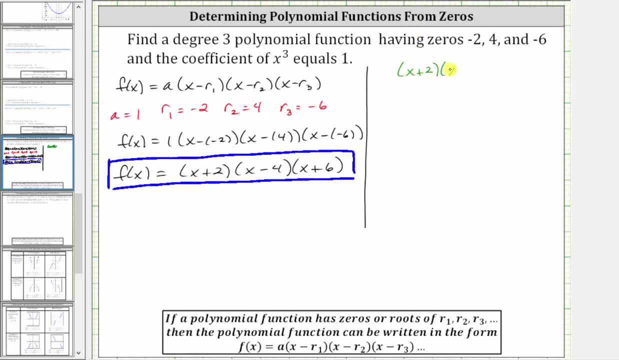 We have the quantity x plus two times the quantity x minus four times the quantity x plus six To determine the product. let's multiply the first two binomials. When multiplying the first two binomials, we have four products. We distribute each term in the first binomial into the second binomial, which means the first two products will be these two products here. 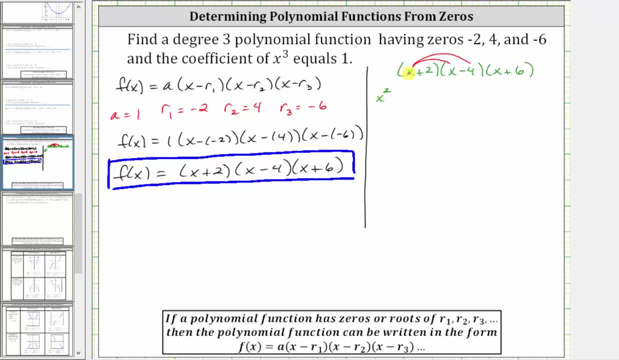 x times x is x squared x times negative four gives us minus four x. And then we distribute the two: Two times x gives us plus two x, and two times negative four gives us minus eight. All this is still multiplied by x plus six. 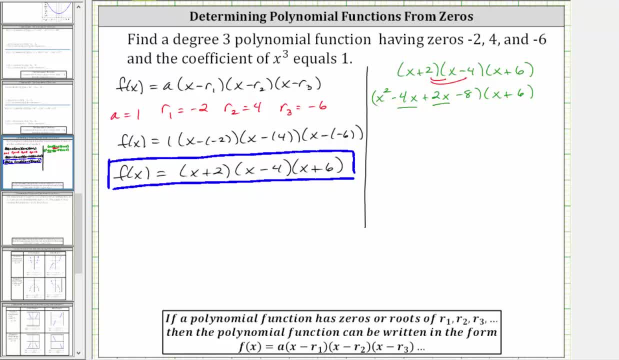 Let's simplify here: Negative four x plus two x is negative two x, giving us the quantity x squared minus two x minus eight times the quantity x plus six. and now we multiply the trinomial. We multiply the trinomial and the binomial by distributing each term of the trinomial.